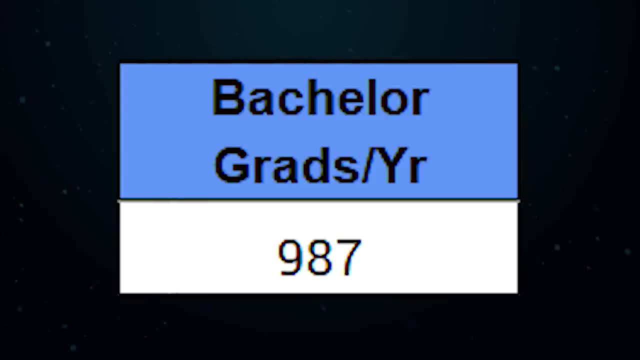 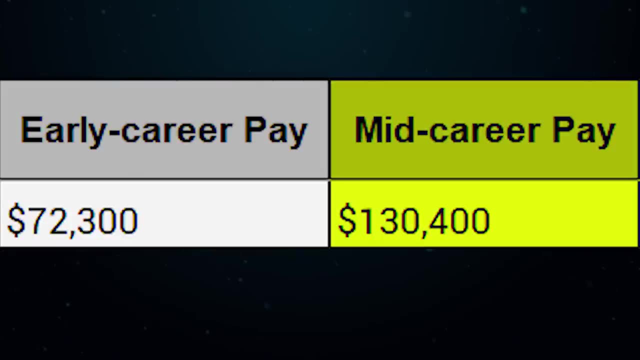 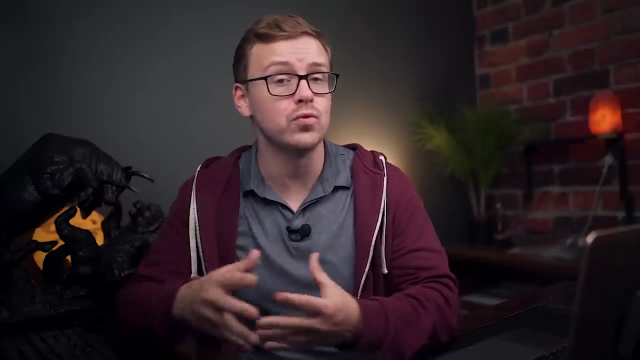 year. This one has about a thousand graduates per year. at the bachelor's level, The early career pay is about 72,000 and mid-career pay is going to be 130,000.. So fantastic salary there. Unfortunately, when it comes to the demand, not nearly as good, And I think the reason for that is because systems 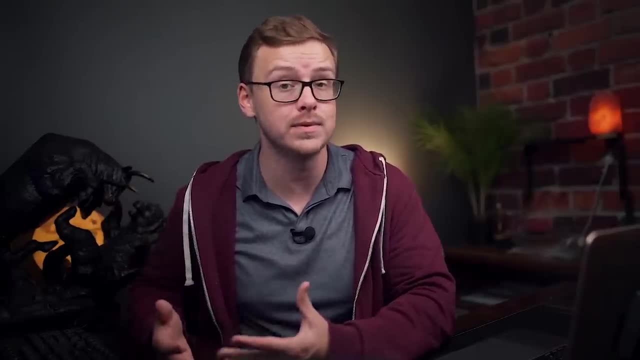 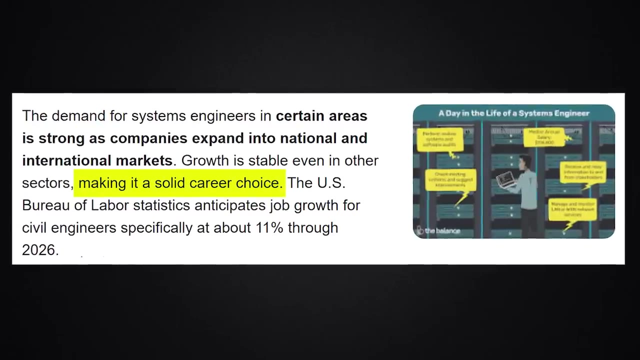 engineering isn't as well known as a lot of other different types of engineering degrees. Now systems engineering as a career is getting more and more popular, So I am very bullish on the future of this degree. So the number of jobs that had the keyword systems engineering degree. 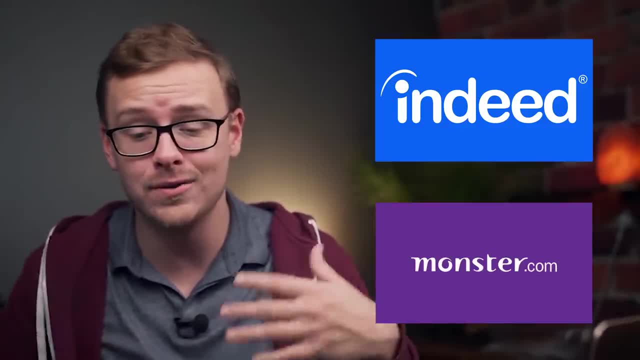 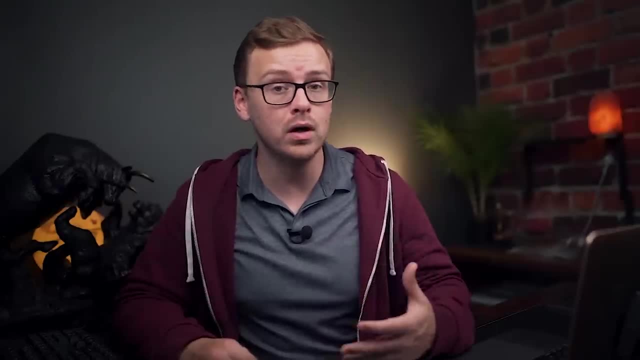 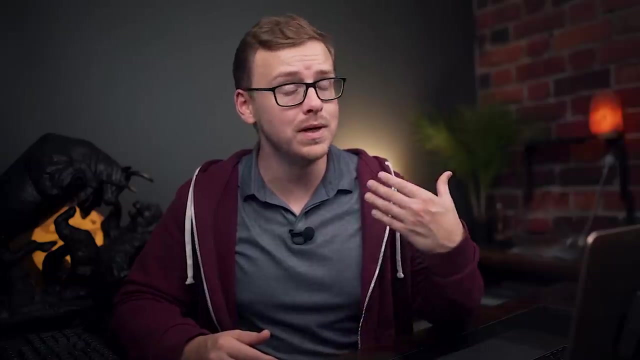 on, indeed, and monstercom were not very high. It was about 127.. And so the demand score is 14.51, which is relatively low, but overall, uh, this is still a very good degree, And when it comes to engineering degrees, I'm going to put this one in B tier, but, like I said, this could be. 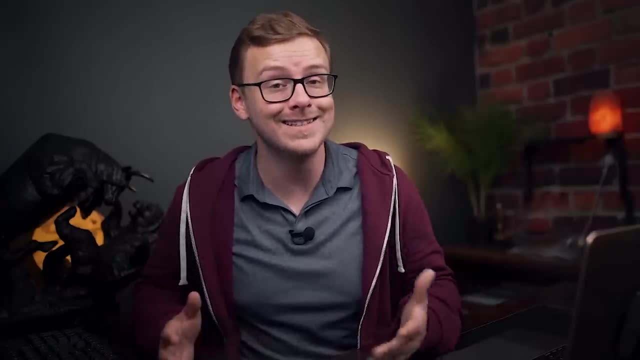 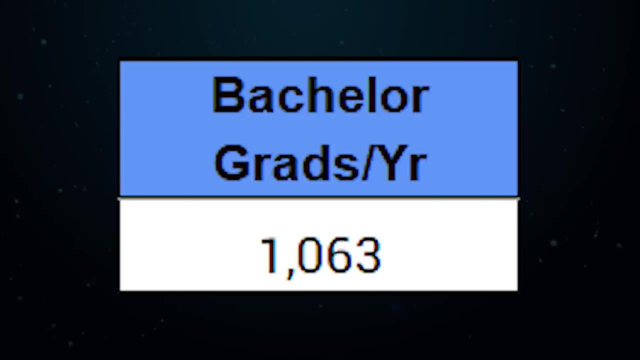 an underrated degree. So I'm going to put this one in B tier. So I'm going to put this one in B tier. It could be a dark horse candidate and I could see this one getting higher in the future. Next on the list is going to be a relatively rare one. Uh, you do see about a thousand graduates per year. 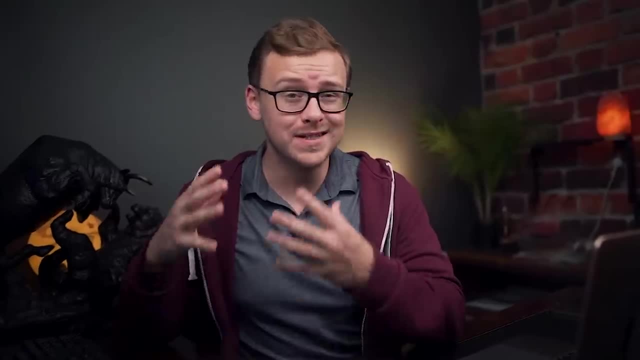 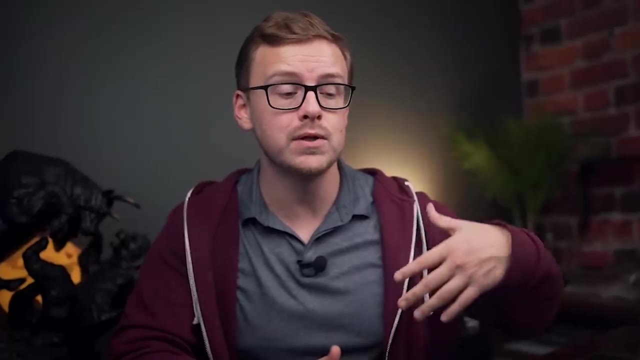 and that is going to be agricultural engineering. uh, very specific, very niche degree. Uh, when it comes to engineering degrees, you really don't need to get too specific with them, because they're already so good on their own that you don't need to specialize as much. but you see, a early career. 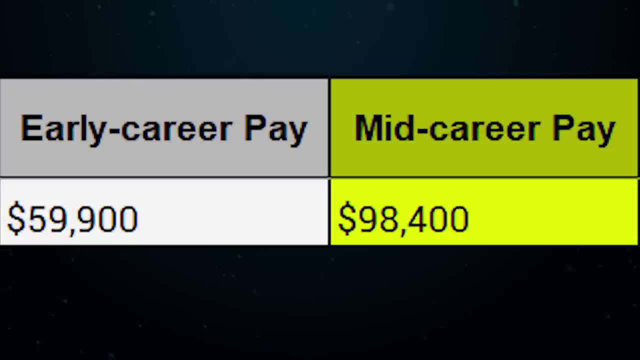 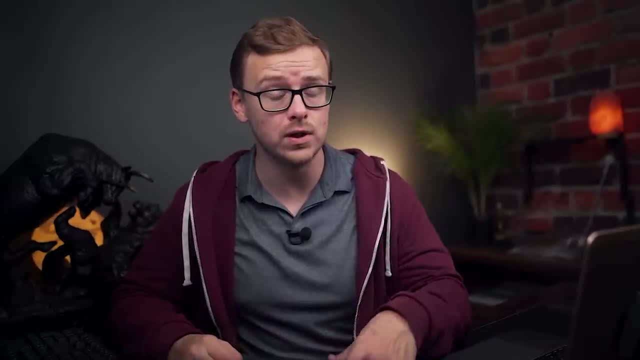 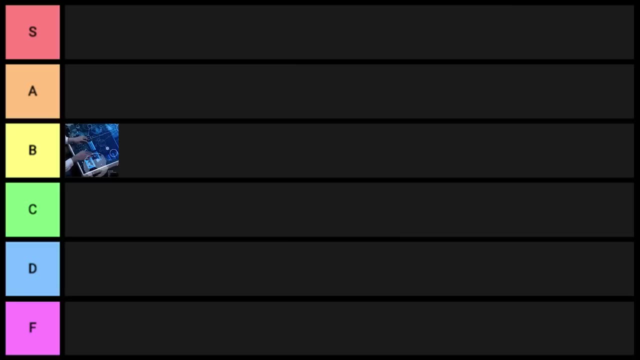 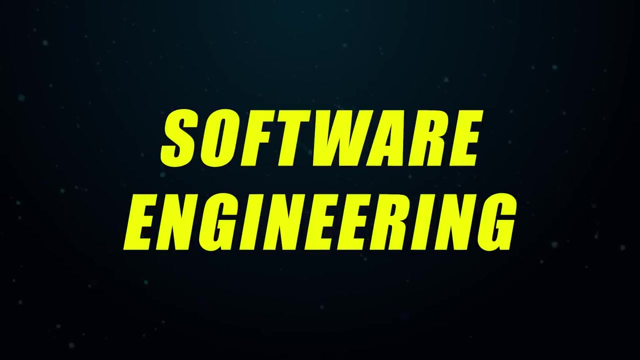 pay of $59,000 a year and mid-career pay is going to be about 13,000.. So that's going to be a very good degree. Next one on the list is going to be software engineering- One of the best overall. 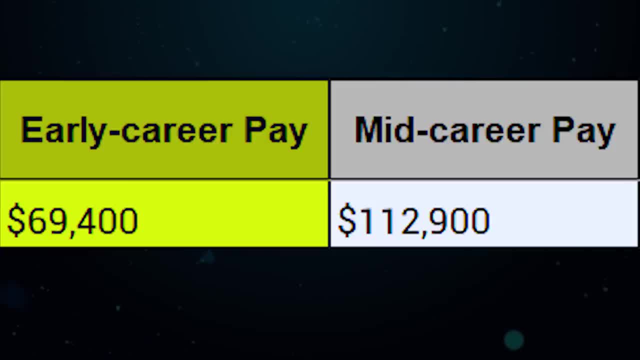 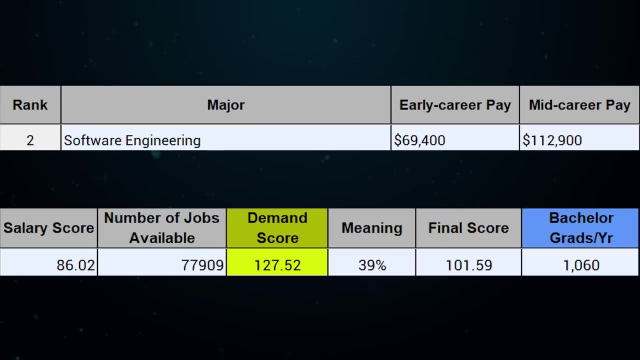 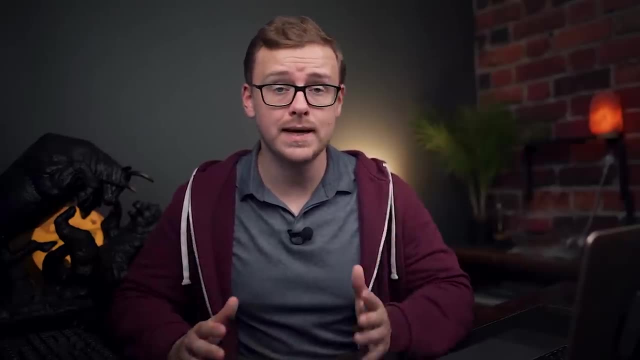 degrees. early career pay is going to be 69,000 a year, Mid-career pay is going to be 112,000.. And the demand score is absolutely ridiculous at 127.. That is the highest demand on the entire list for engineering degrees. So yeah, this is a fantastic one. Clearly, this one goes in S tier. 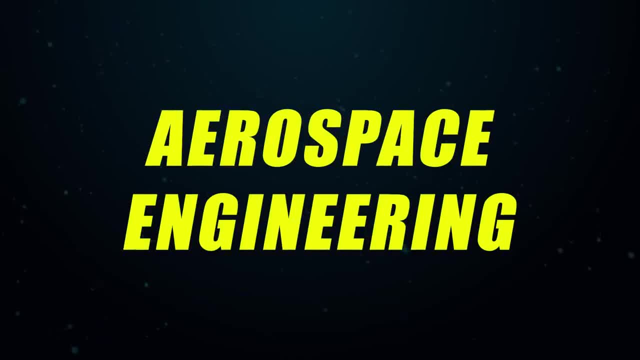 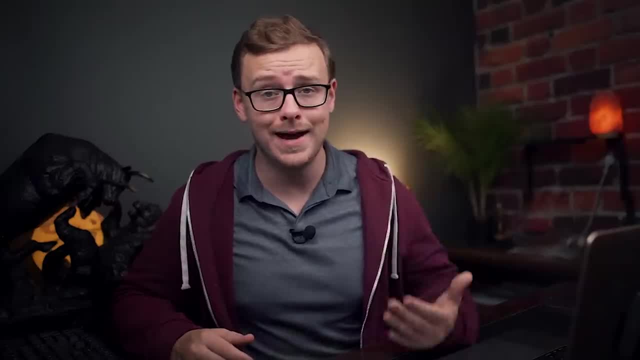 Next one on the list is going to be aerospace engineering. Uh, aerospace aeronautical industry in general took a huge hit during COVID And I did say in videos I've made in the past that this is one of those industries that can be a little bit boom or bust, but you're going to start off. 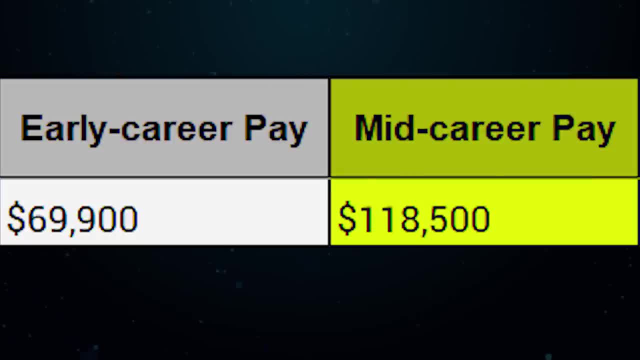 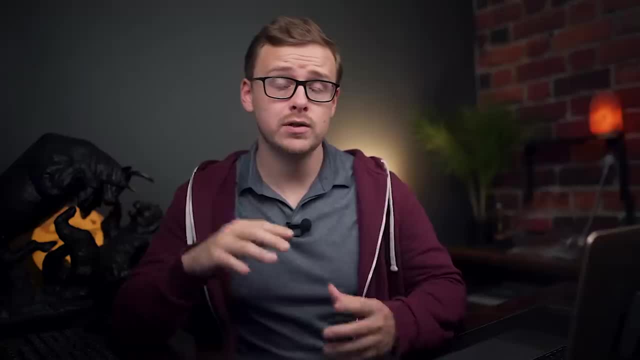 about $69,000 per year, and mid-career pay is 118,000.. There's about 4,000 graduates per year and the demand score came out to be about a hundred. So yeah, this one's pretty good Uh. 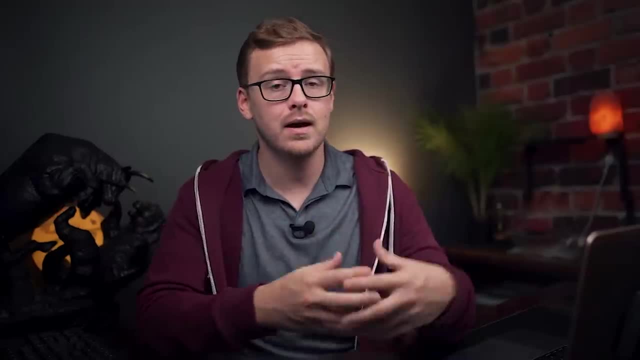 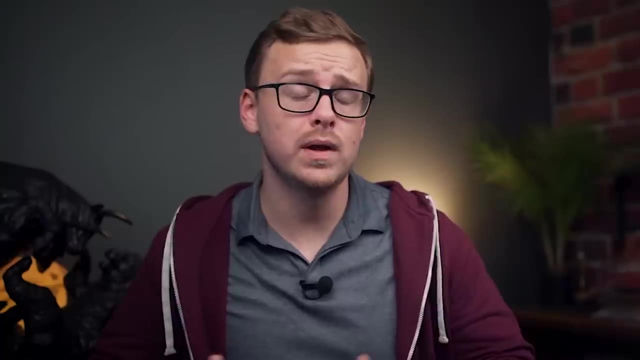 the only problem is is it's, you know, relatively specific Um, and you're going into an industry that can be boom or bust, And so for that reason, I'm going to go ahead and put this one into a tier. Next one on the list is going to be architectural engineering. with less than a 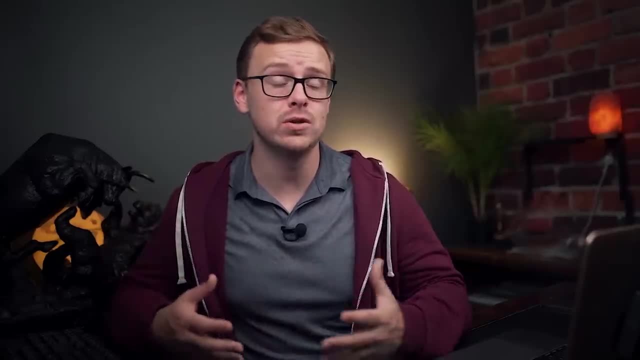 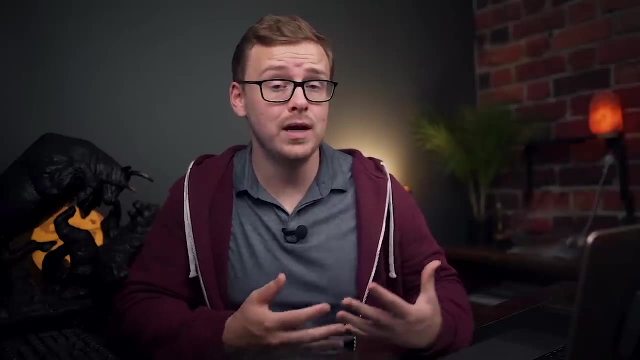 thousand graduates per year. Very specific, very niche degree And I'm going to go ahead and put it into D tier: Early career pay: 61,000. mid-career pay is 97,000 a year. That is relatively low pay. 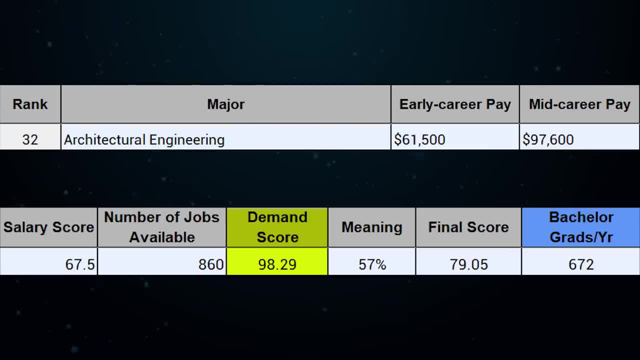 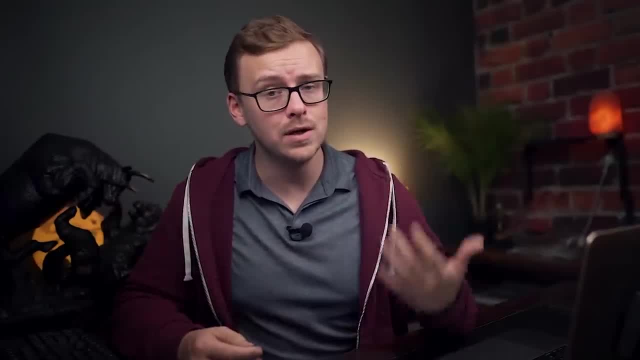 for an engineering degree, The demand score is pretty good at about 98.. However, overall, because of the fact that it is so specific and the pay is a little bit low when you're comparing it to other engineering degrees, it's not that great. It's not horrible either, So for this one I'm 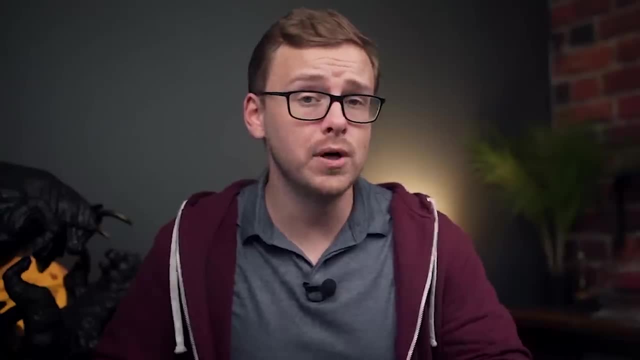 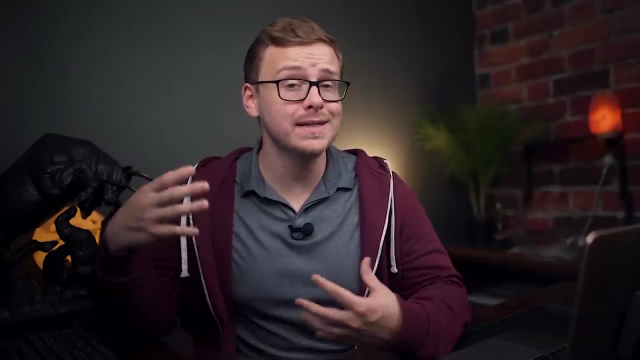 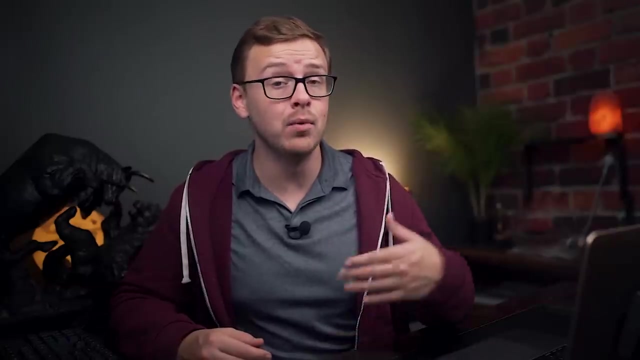 going to go ahead and put it into D tier. Next one on the list is going to be biomedical engineering. This one has almost 7,000 graduates per year, And this is one that I put as a dark horse candidate when I made my very first video on engineering a few years back, And ever since then, the more 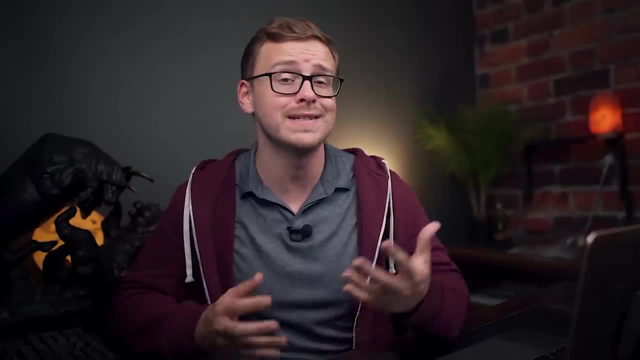 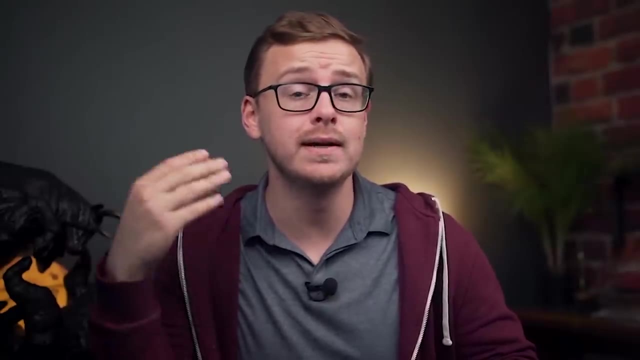 I've studied it, the more I've looked into it, the statistics, the trends, et cetera. it does seem to be on an upward trajectory. Now, one thing that really stands out about this one is the meaning score is much higher than other types of engineering degrees, So it's 71%. 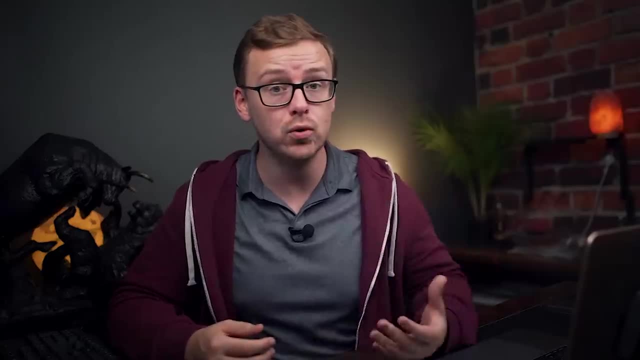 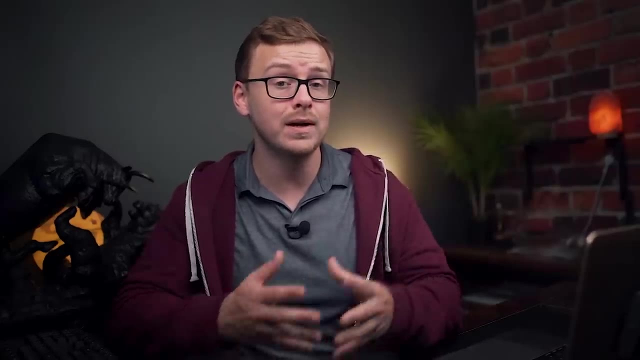 most engineering degrees are usually in the 50s, So that means people who like biomedical engineering really like biomedical engineering, And it also means that you're likely going to end up in a career that is extremely meaningful, And so, over a long period of time, you're probably 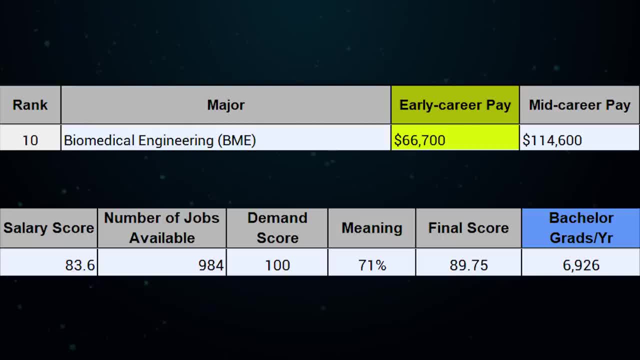 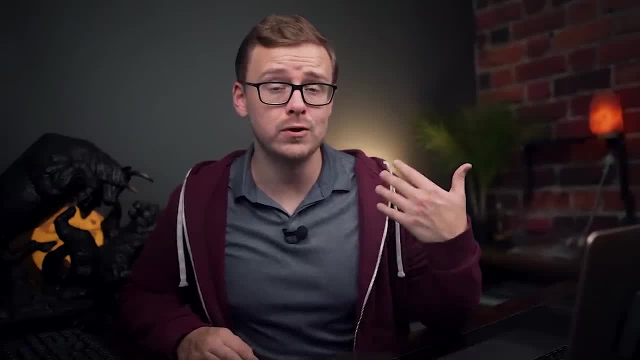 going to be a little bit happier with it. So the early career pay is going to be 66,000 and mid career is about 114,000.. So, yeah, this one pretty solid If you're somebody who is interested in kind of the combination of, like health and engineering. 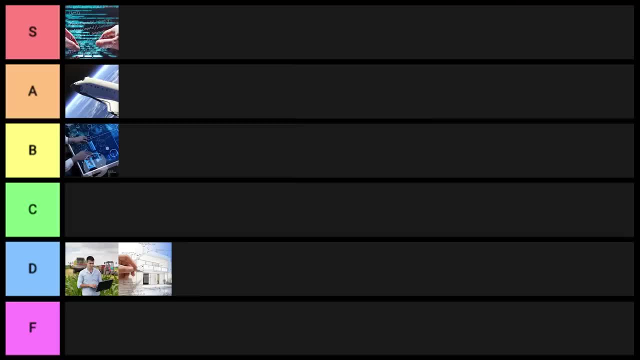 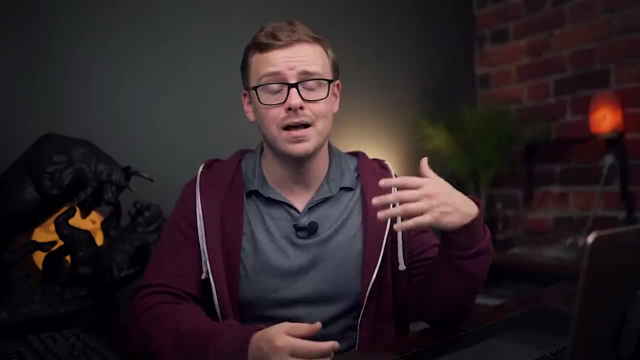 you know, combined together, this is a good one for you to look into. I'm going to go ahead and put it into B tier. The only reason it isn't higher is because, again, it's just so specific. A lot of the time if you get like a mechanical engineering degrees you can still apply to. a lot of the same jobs as people with biomedical engineering degrees, And so, especially when it comes to engineering degrees, I think flexibility is key. Next one on the list, at about 10,000 graduates per year, is going to be chemical engineering. One of the most important things about chemical engineering is that it's going to be a lot of. 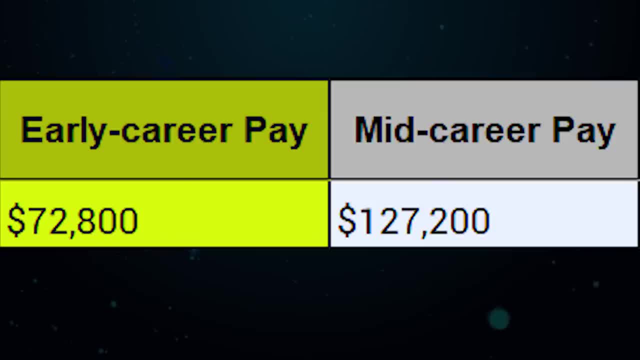 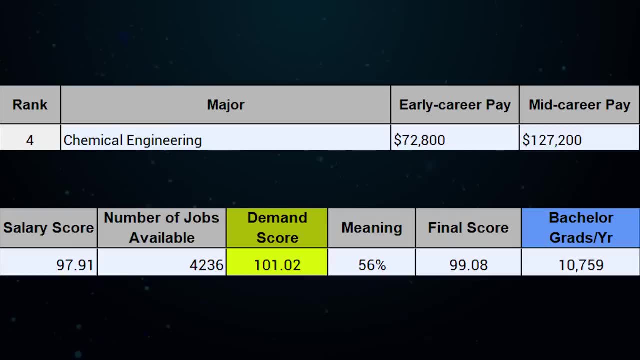 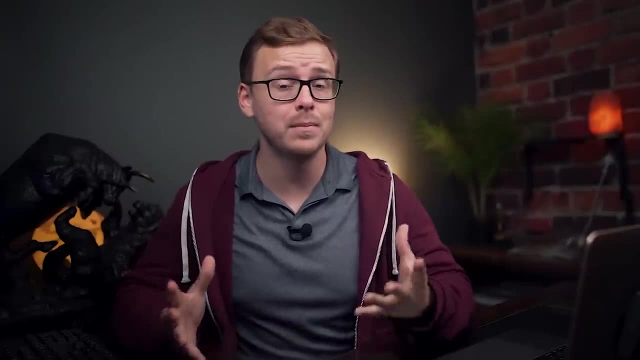 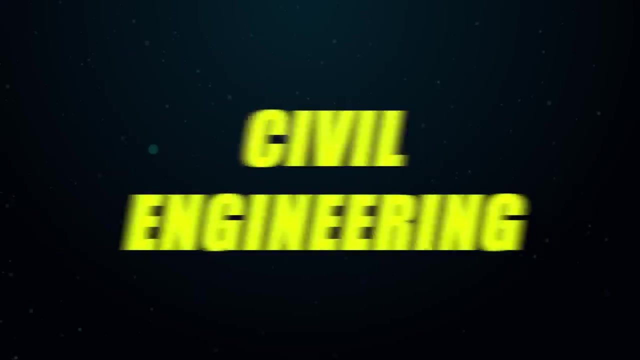 engineering degrees. So, yeah, this is a pretty good one. Doesn't quite make it into S tier status just because it doesn't pop off the page, but very solid choice overall. I'm going to put this one into A tier. Next one on the list is going to be civil engineering, with about 13,000 graduates. 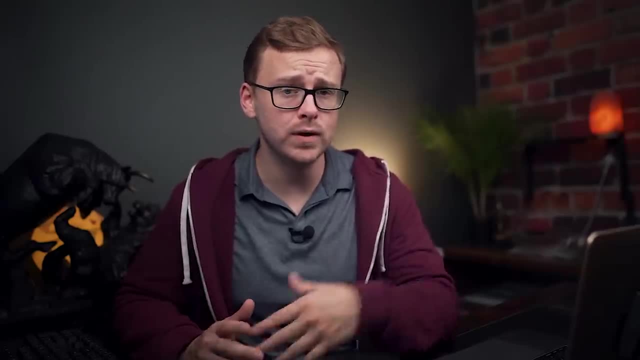 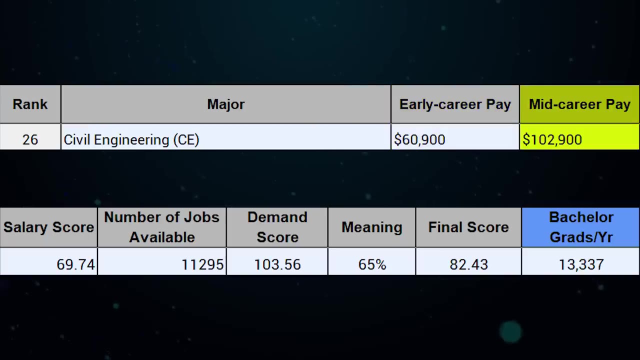 per year. This one also has a relatively high degree rate, but it's going to be a lot of high meaning score. That's kind of one of the outliers with this one. It's about 65%. Early career pay: $60,000 a year. Mid-career pays about $102,000, which is good when you compare it to. 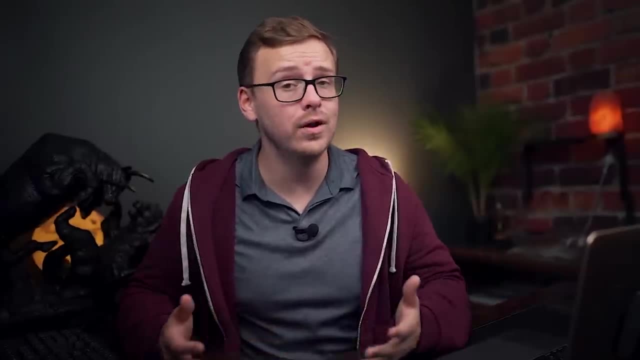 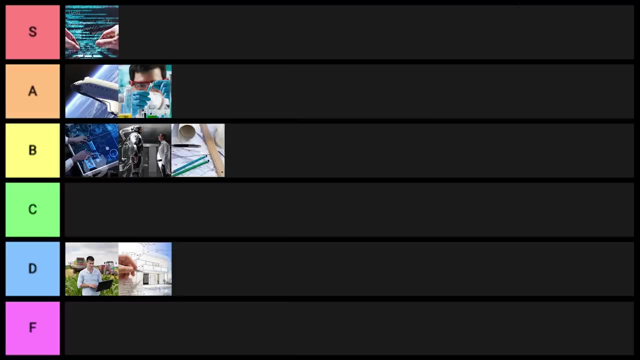 all types of degrees, But for engineering degrees specifically, it's not all that impressive. So yeah, again, another very solid choice Doesn't pop off the page. I'm going to go ahead and put this one into B tier. Computer engineering is going to be next, And this one has about. 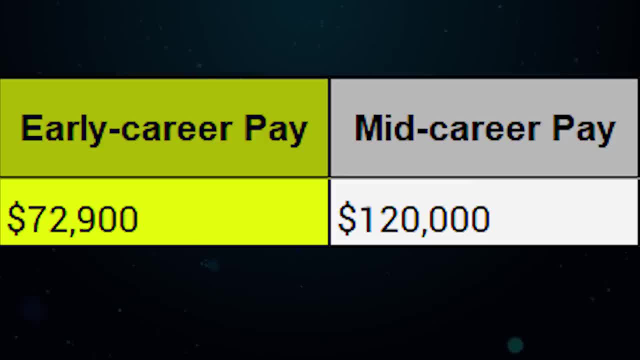 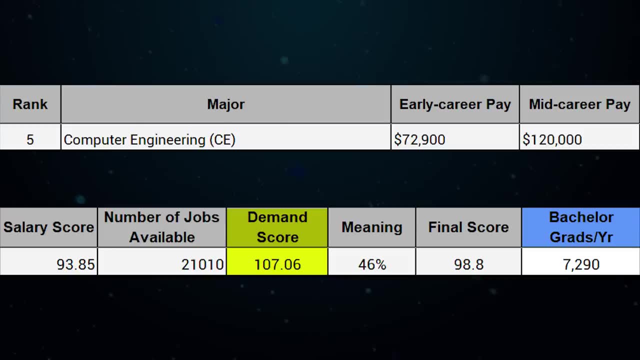 7,000 graduates per year Start off about $72,000 a year and mid-career pay is going to be about $120,000.. This one has a very good demand score as well, at about 107.. So basically everywhere you. 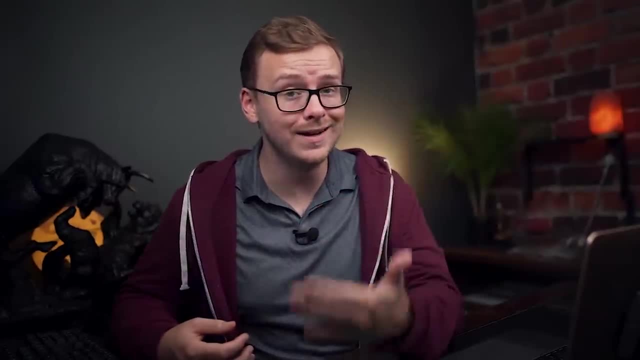 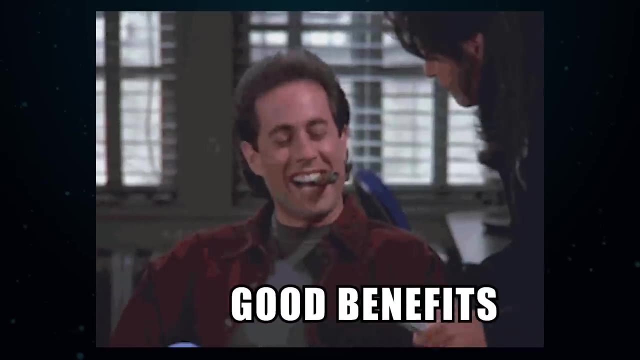 look, really good pay, really good demand. You're going into an industry that tends to also not only just pay you really well, but you get bonuses, you get stock options, you get really good benefits, tons of opportunity in the technology industry. So yeah, computer engineering, another one that. 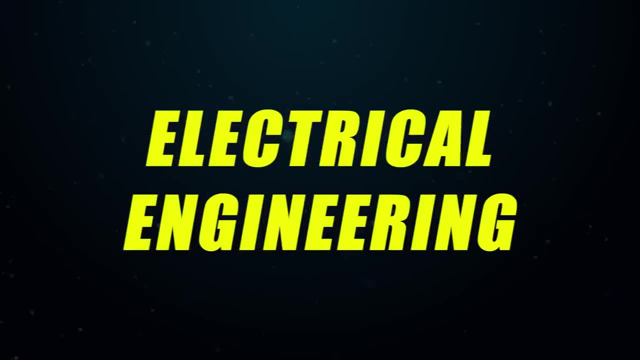 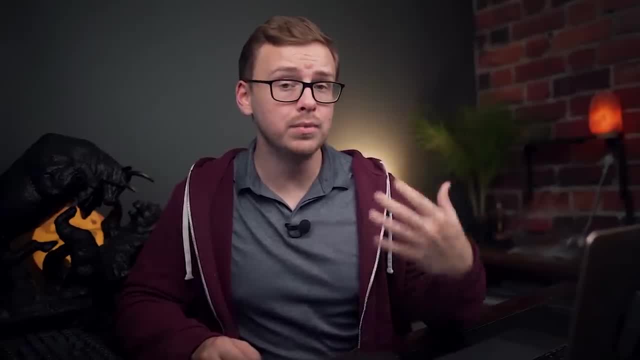 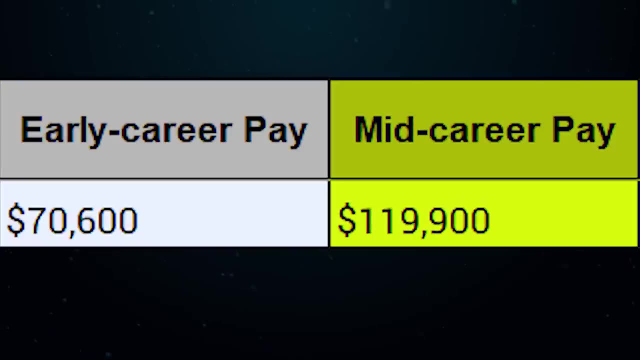 is clearly S tier. Next one on the list is going to be electrical engineering. Interestingly enough, most identical stats, just slightly lower than computer engineering everywhere you look. So early career pay is going to be 70,000 a year. mid-career pay is 119,000.. So you know slightly. 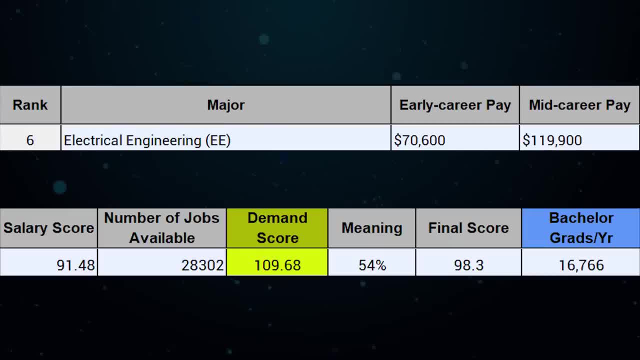 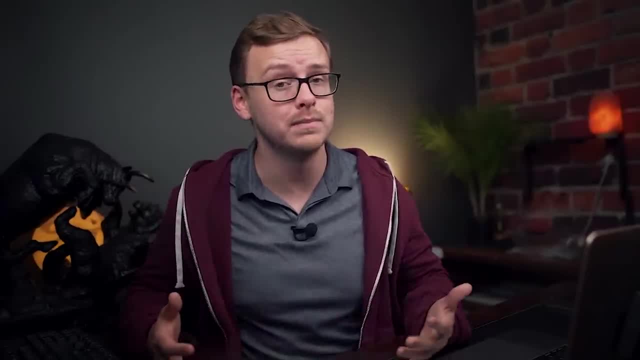 lower. However, the demand score is going to be just a little bit higher, And the great thing about electrical engineering is it isn't as specific as computer engineering, So you're going to have a lot more flexibility. So electrical engineering is another one where I'm going to 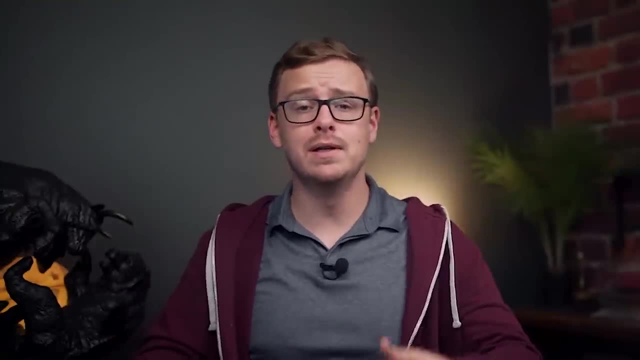 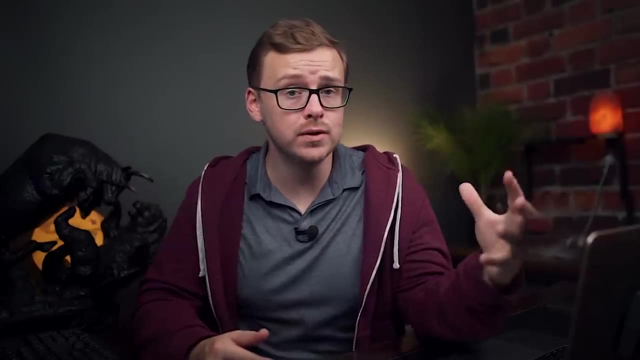 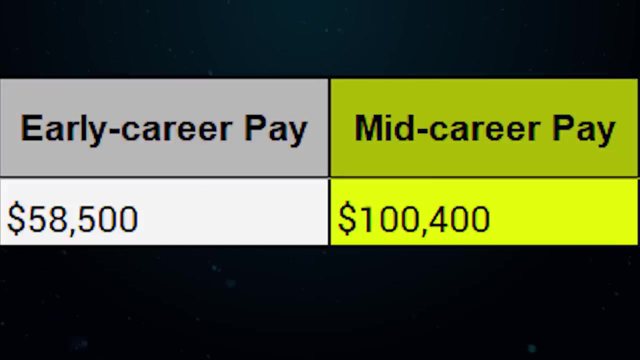 actually put this one into S tier. The next one on the list is going to be electrical engineering. Now, when it comes to the pay, this one is going to be relatively low when you compare it to other types of engineering degrees. Early career pay is 58,000, mid-career pay is about $100,000 per year. 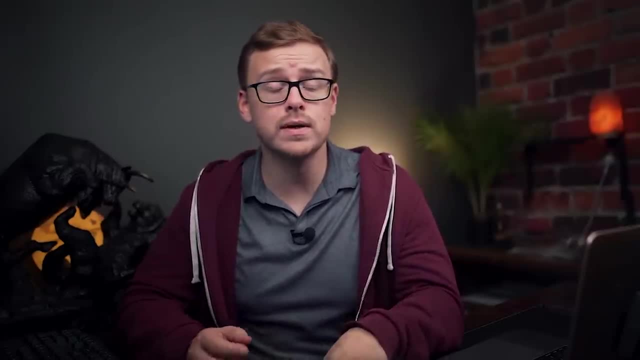 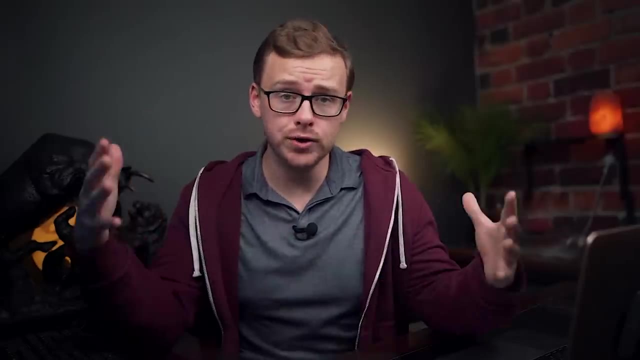 Now, when it comes to the demand, relatively good. The demand score is about 100.. And also the meaning is relatively good as well, about 63%. So if you compare this to like all degrees, pretty good. But when it's on a list of other engineering degrees, 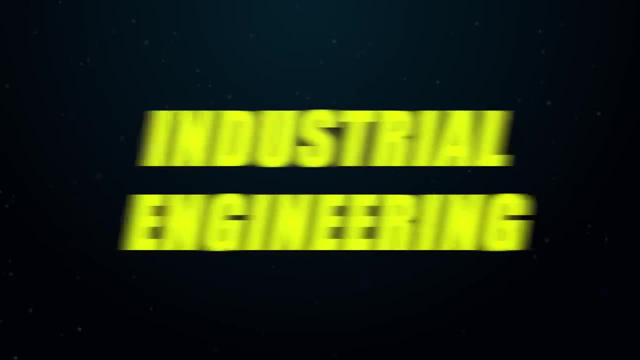 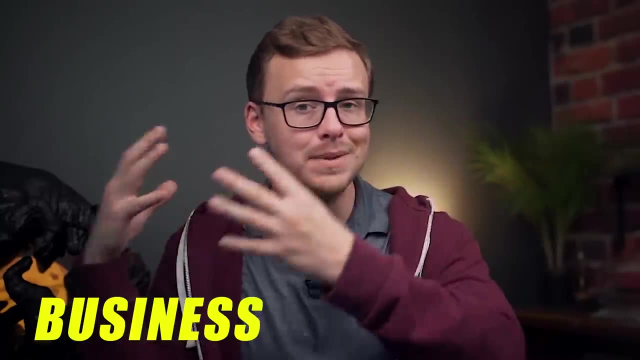 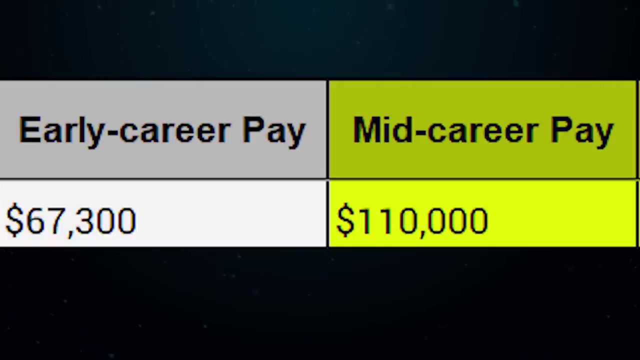 it's going to be C tier. Next one on the list is going to be industrial engineering. This is one of my favorite ones because it's so flexible. It's basically like business combined with engineering. So you're going to start off about $67,000 a year. Mid-career pay is 110,000.. 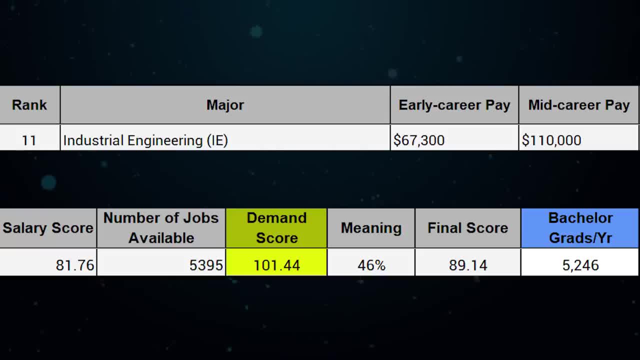 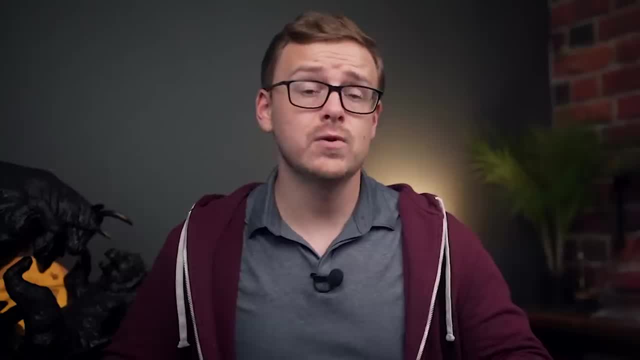 And then the demand score here is going to be 101, which is pretty good as well. And then on top of that, like I said, it's very flexible, And for that reason I'm going to go ahead and put this one into A tier. Next one on the list is going to be marine engineering. So if you're going to be, 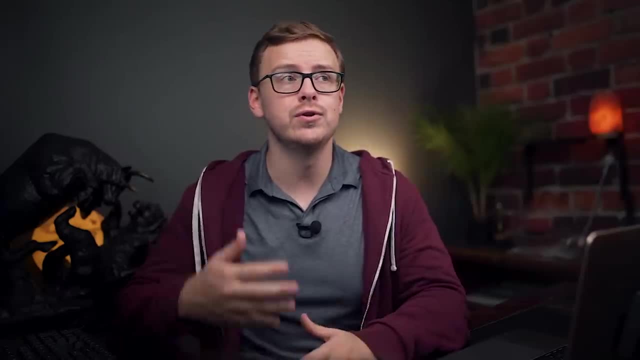 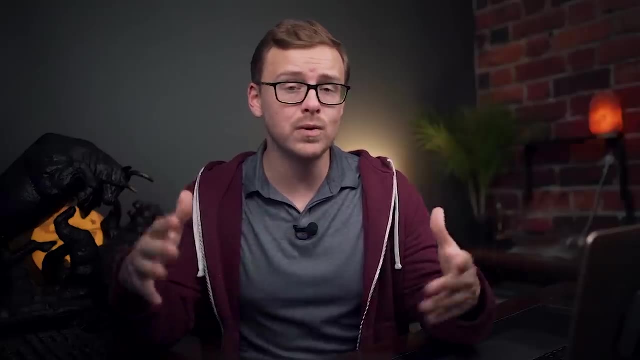 engineering, and this one is very similar to environmental engineering, where it has some benefits here and there. but the big reason why it's not going to make it into the higher tiers is because it's just too specific, too niche. So your early career pay is going to be about. 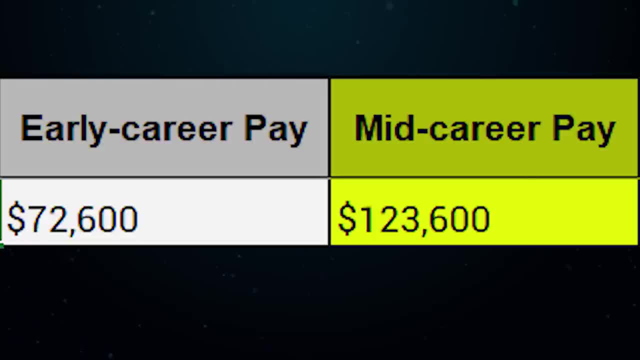 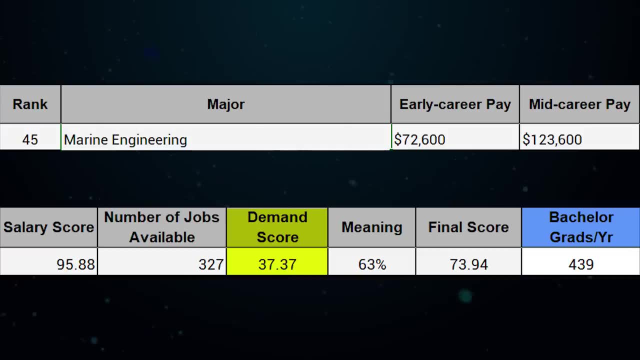 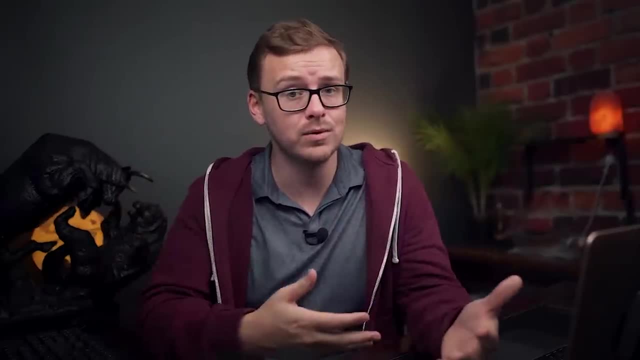 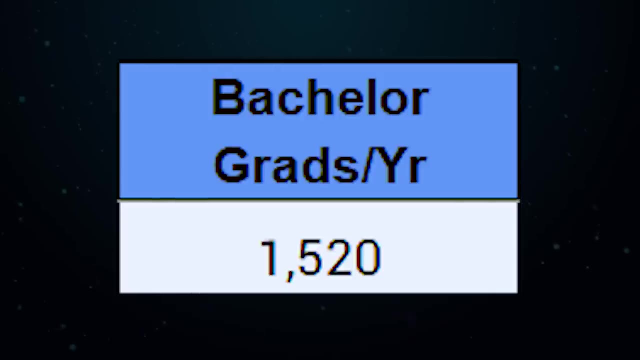 it into the higher tiers. So you're going to have to make it into the higher tiers, And then, on top of that, it's not very flexible, And so for that reason, I'm going to have to put this one into C tier. Next one on the list, with about 1,500 graduates per year, is going to be materials. 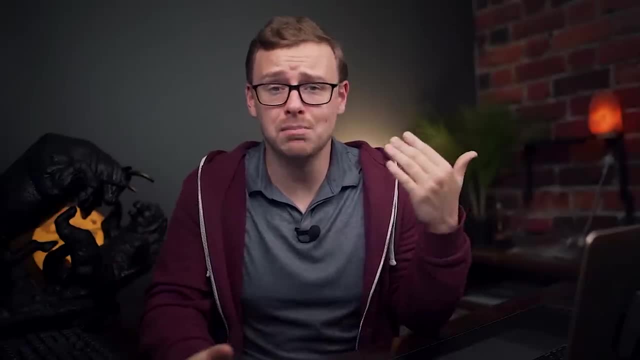 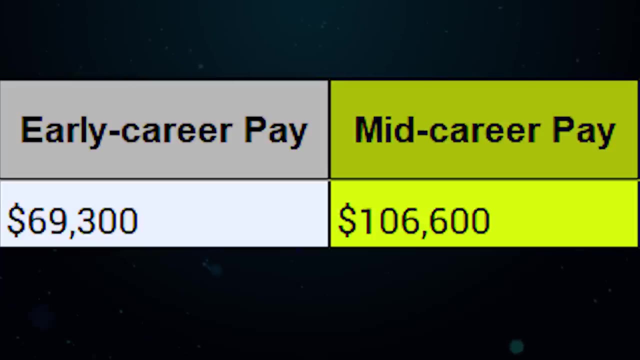 engineering. Now this one is pretty mediocre across the board, especially when you're comparing it to other engineering degrees. Early career pay is 69,000.. Mid-career pay is 106,000.. The demand score is 53.. The meaning score is relatively low at 47.. It's also not a super. 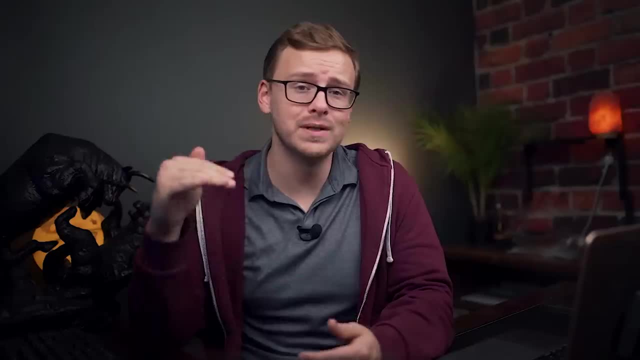 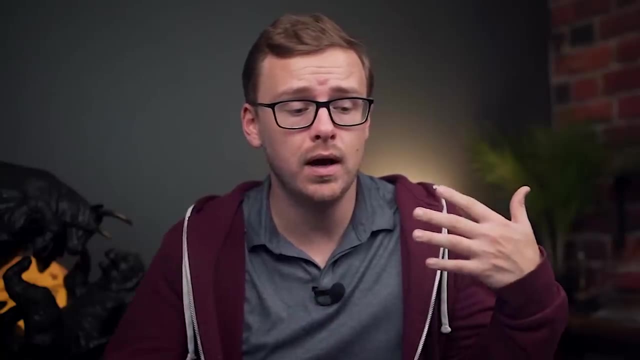 flexible degree either, And so, like I said across the board, it's either middle or even below average. But, with that being said, very cool. A lot of cool stuff is coming out that are applications of materials, engineering. There's material coming out, for instance, where it can. 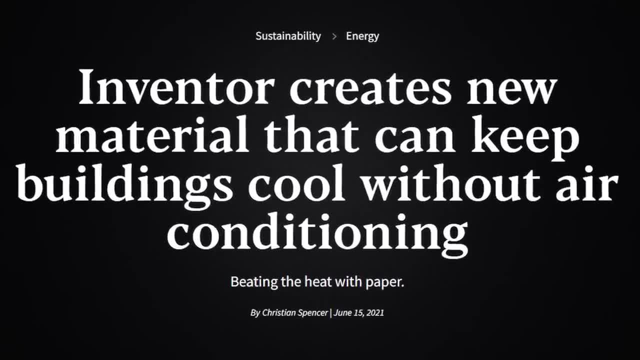 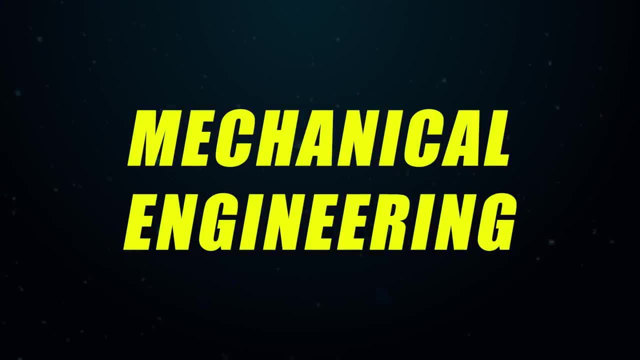 keep your house cool without even using air conditioning, which is super cool. But yeah, overall on this list, I have to put it in D tier. Next one on the list is going to be mechanical engineering: Very flexible degree. That's the biggest positive about mechanical, Also one of 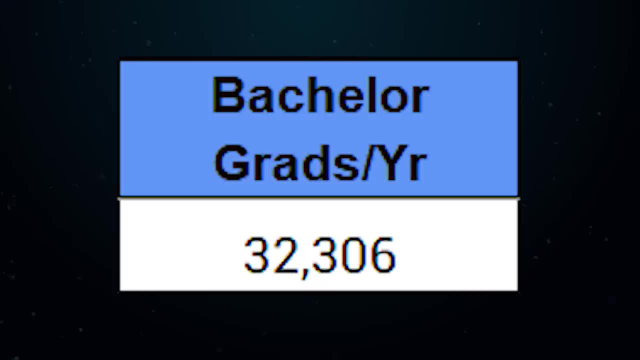 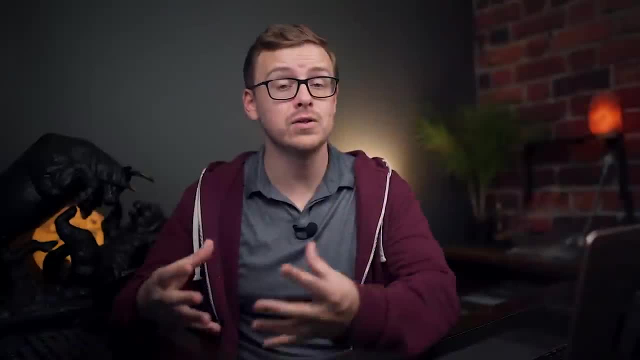 the most common engineering degrees, if not the most common, at 32,000 graduates per year, And one of the big things about having a lot of graduates is it's almost like the degree itself has its own brand name, And if you know anything about brand names with companies and that sort of thing, 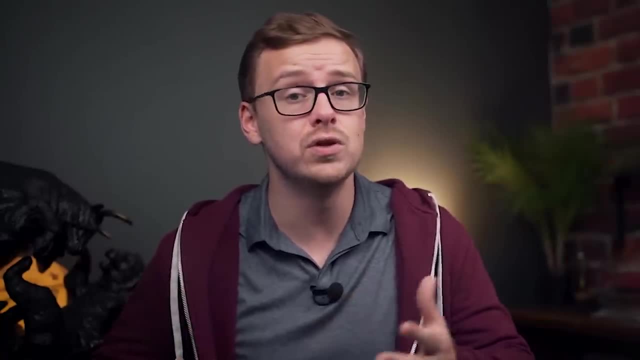 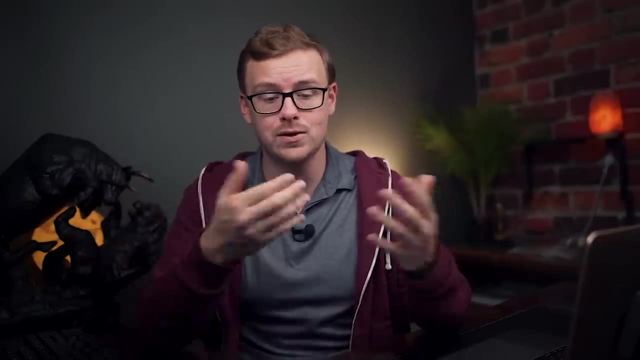 you know, you probably think it's not all that important, but it actually makes a huge difference. If somebody sees a mechanical engineering degree, they're going to be like engineering degree, And then they see some random degree like actually the next one, we're 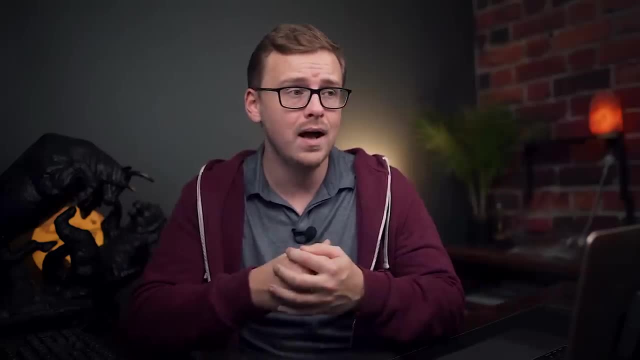 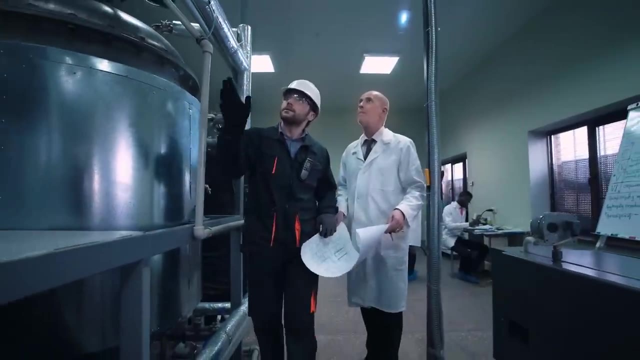 going to talk about on the list, which is, you know, mechatronics, A lot of the time they recognize mechanical engineering. They've probably hired people with mechanical engineering degree. They've worked with people with this degree And so they sort of have some familiarity with it. They kind 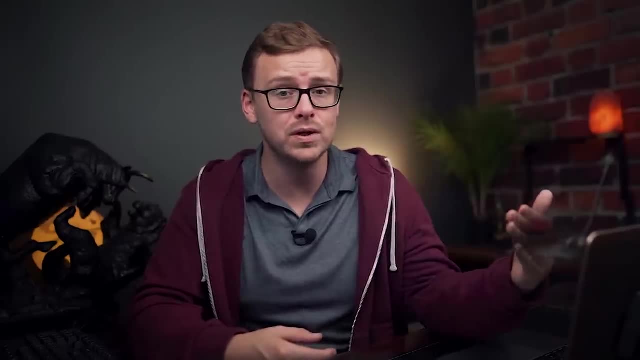 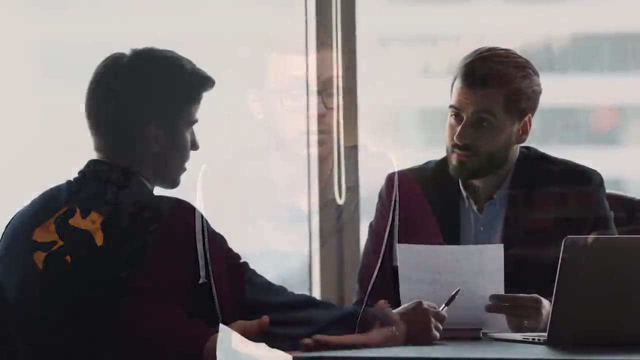 of know what they're going to get. But when it comes to these very specific, very niche degrees where there's maybe not a lot of graduates, it could be just as good, maybe even better, in terms of the education you get. You could be much more knowledgeable on certain things, But unfortunately, just because of the fact that, 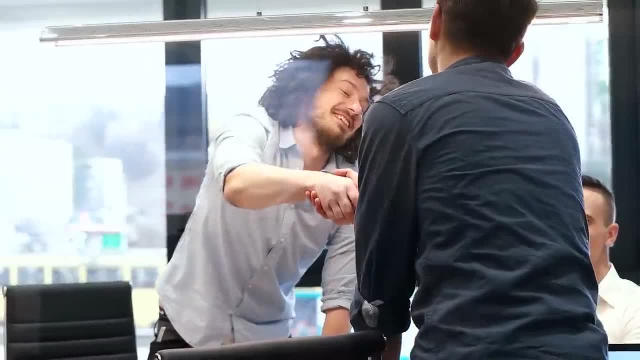 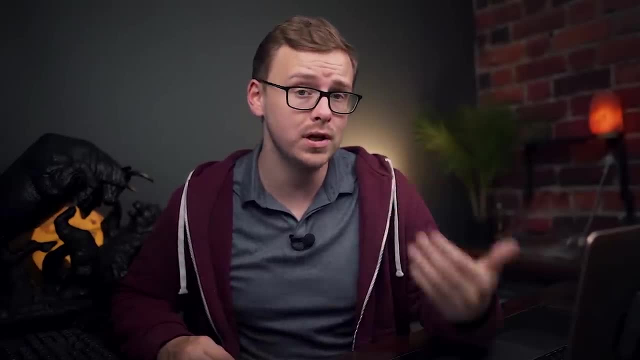 people don't recognize the degree a lot of the time. they're going to go with the one that they know and recognize. But with that being said, very solid stats across the board. for mechanical engineering, Early career pay is $66,000.. Mid-career pay is $110,000 a year. The demand: 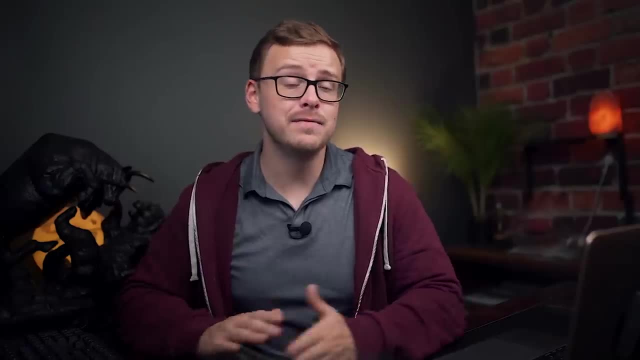 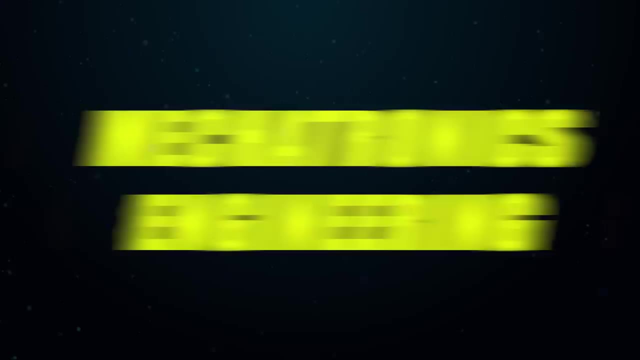 score is super solid at $105,000.. And it's a very flexible degree. So, yeah, this one is going to go into A tier. The next one on the list, the one I just mentioned, was mechatronics engineering, And this is a super 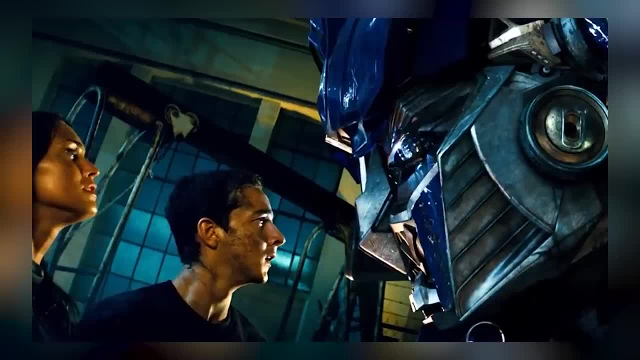 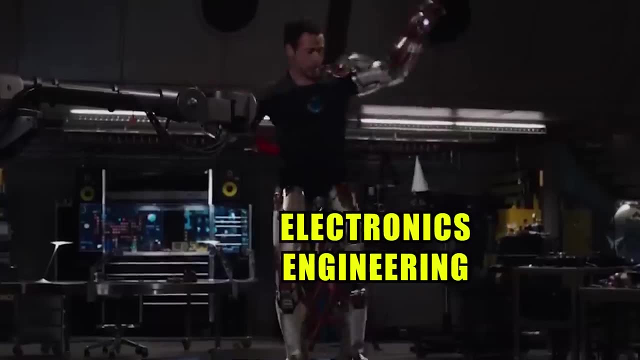 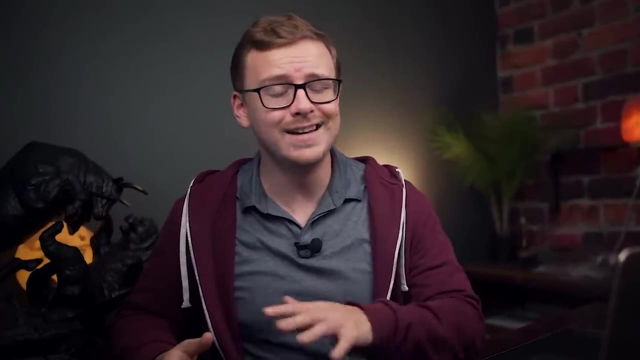 cool, relatively new type of engineering that focuses on robots. So basically it's kind of a combination of mechanical engineering, electrical engineering, electronics engineering as well as robotics. Super, super cool degree. A lot of great things you can do with it. Not nearly as well. 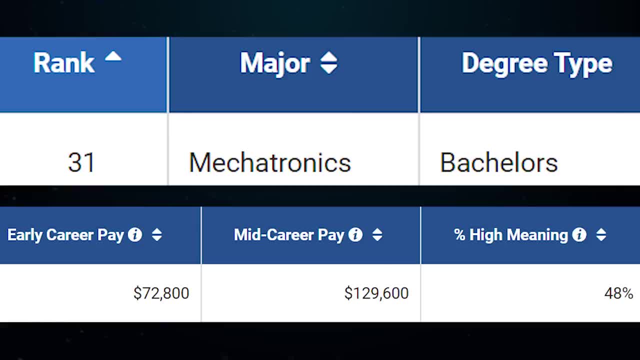 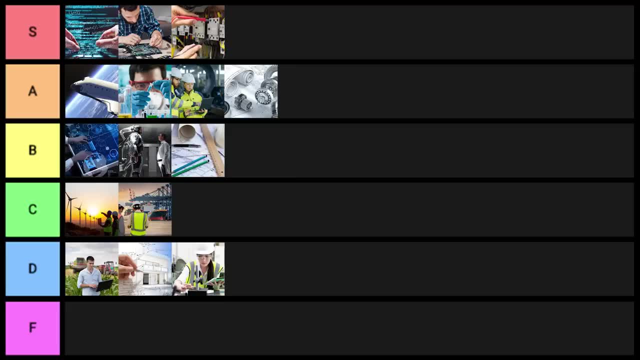 known as some of the other ones. However, with the statistics- I've looked up on it- it is extremely solid, And so for that reason, I'm going to just barely barely put it into A tier. It just squeaks into A tier. Next one on the list is going to be most engineering technology degrees. It seems like 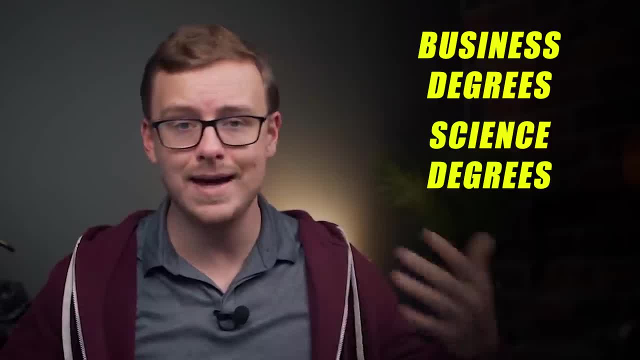 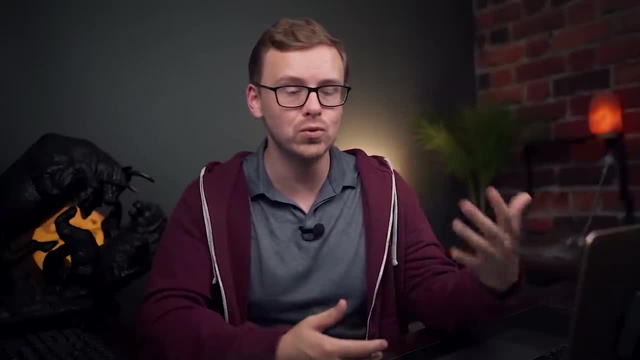 every different degree type- whether you're talking about business degrees, science degrees, engineering degrees, et cetera- has these sort of like grifter type degrees that these schools that want to make way too much money for the value that they're giving A lot of these for-profit. 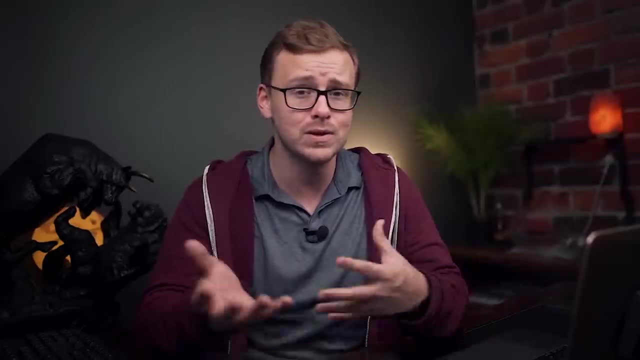 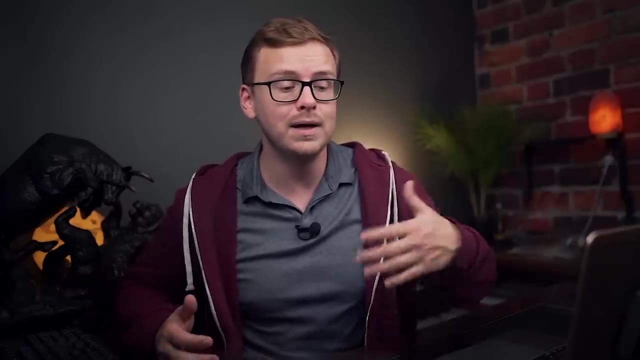 schools, for instance, come up with a lot of these for-profit schools that they're giving, And so to incentivize students to enroll in these different fields and they sound really good, right Like, oh, engineering technology, That sounds amazing, But engineering technology degrees. 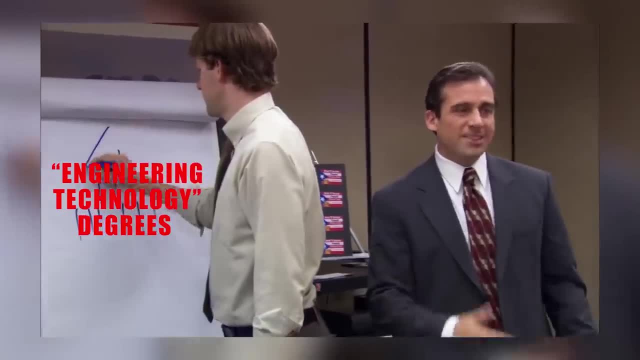 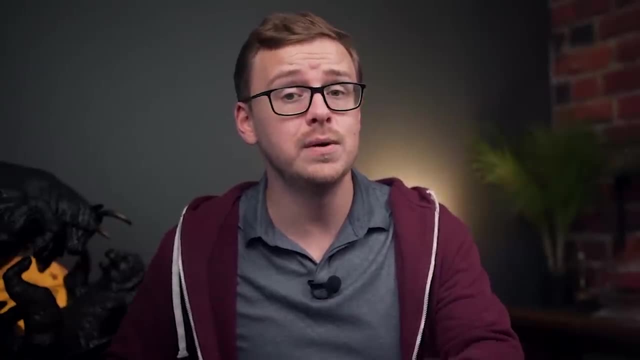 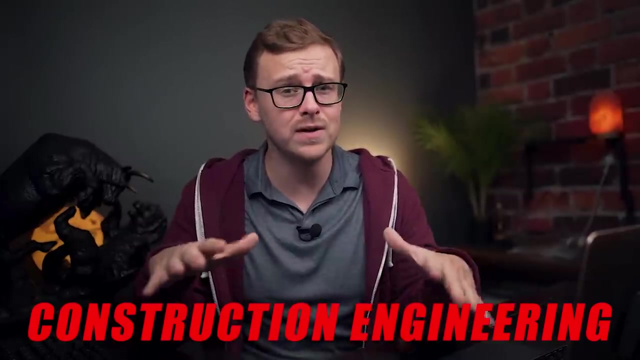 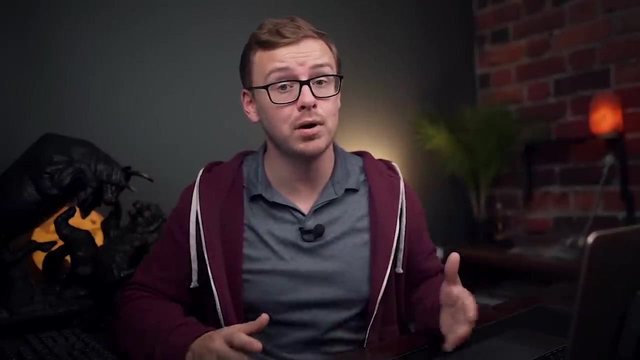 are not technically engineering degrees, It is a. it's not even a scheme per se, It's. So a really good example of this is going to be construction engineering technology. So, first of all, construction engineering technology is even more specific. So that's a big problem right off the. 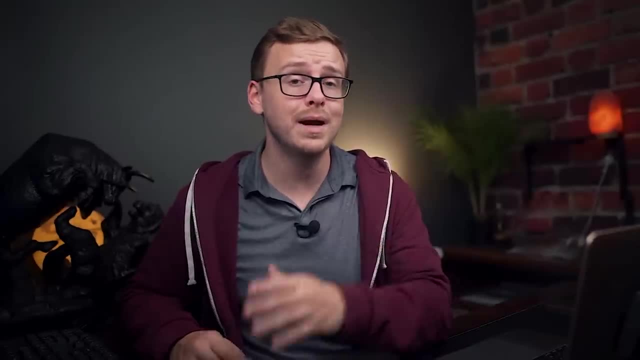 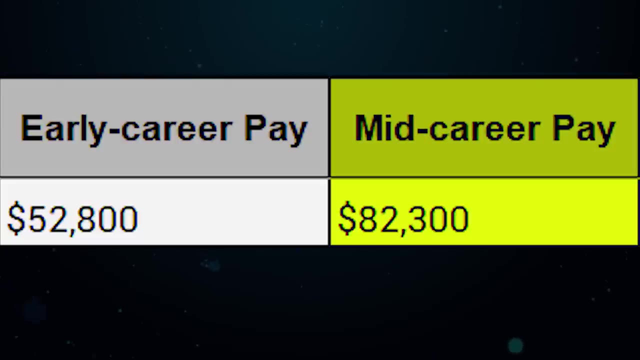 bat. It's not a very flexible degree. On top of that, when you compare it to other engineering degrees and you look at how much they're making, you know early career pay is $52,000 a year. Mid career pay is $82,000.. Not great compared to engineering degrees. And then when you look at 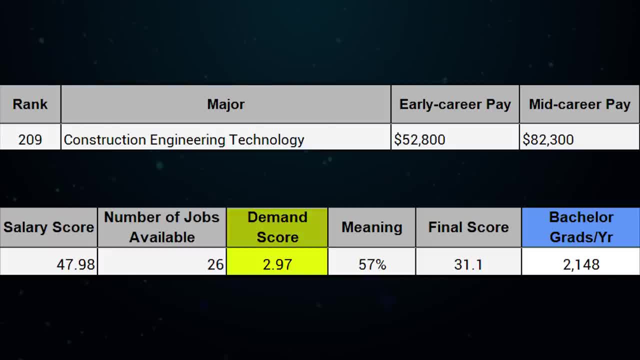 the demand score it's even lower. right, The demand score here is the lowest on the entire list at 2.97.. So some of these engineering degrees are even lower than the demand score here. So some of these engineering degrees are even lower than the demand score here. So some of these engineering 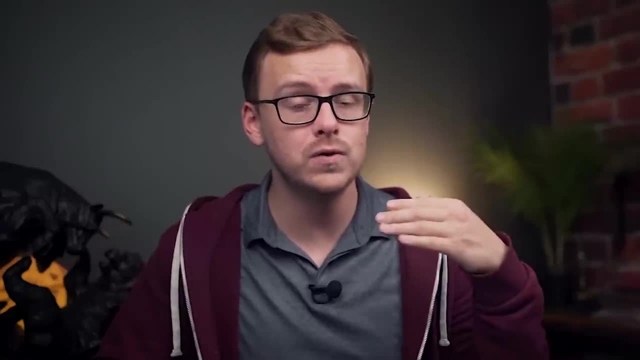 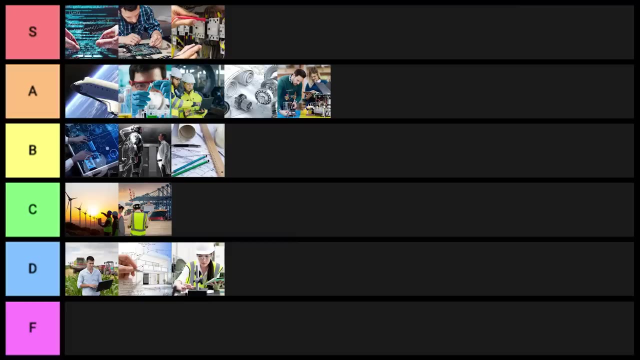 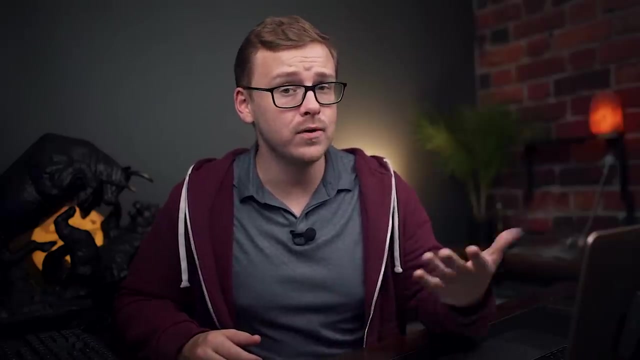 technology degrees can be all right, but I want you to know, because so many people get confused by this, that they are not real engineering degrees. So, yeah, these are going to go into F tier. Next one on the list is going to be network engineering. For this one, relatively low pay for. 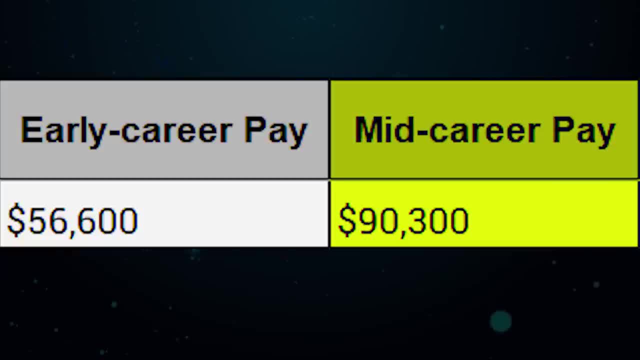 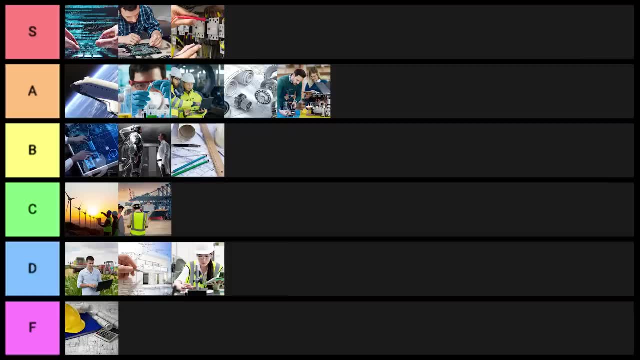 an engineering degree starting off at $56,000 a year and mid career pay is $90,000.. However, the demand score is really good at a solid 100.. So for that reason, this one is going to go into C tier. Next one on the list is going to be nuclear engineering, a relatively rare one. 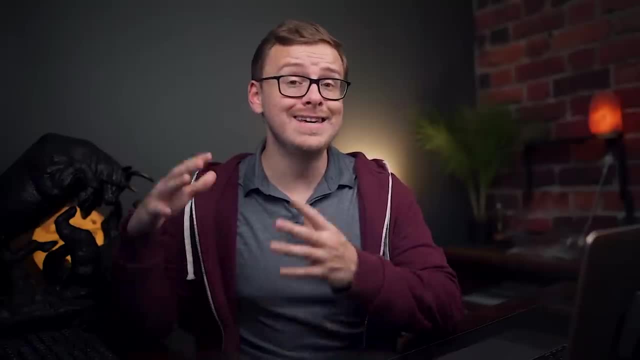 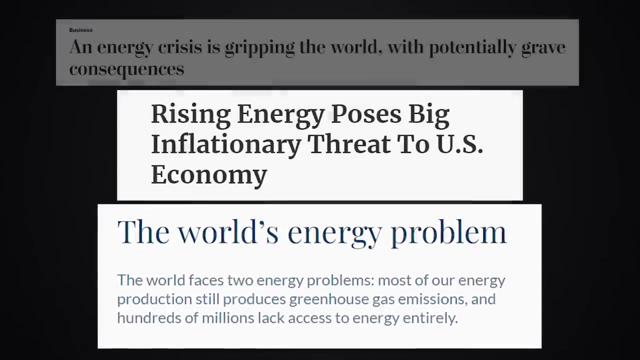 only about 500 graduates per year. Now this one is in the energy industry, which again can be extremely up and down, extremely boom or bust, And we saw during, you know, everything that happened the last few years. the energy industry did take a huge hit. But with that being said, 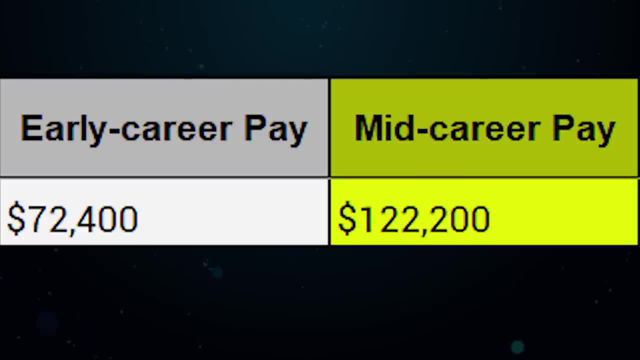 a pretty good pay here: $72,000 starting out, $122,000 mid career. The demand score here is on the slightly lower side at 50%, So this one is going to go into C tier. Next one on the list is: 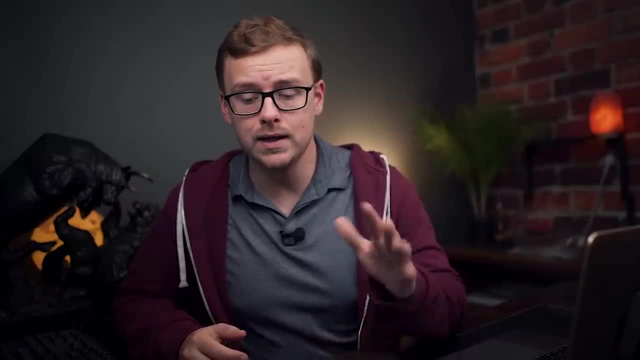 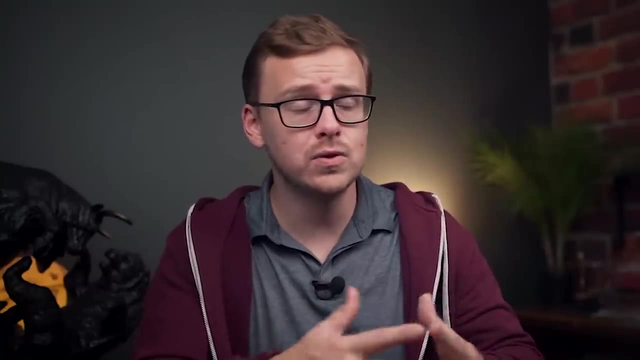 I am a big fan of nuclear engineering, though, and it does have a relatively high meaning score, at about 63%, But there's so many other factors that go into the energy industry that we simply cannot control, And we definitely can't predict certain governments, for instance, like this type of 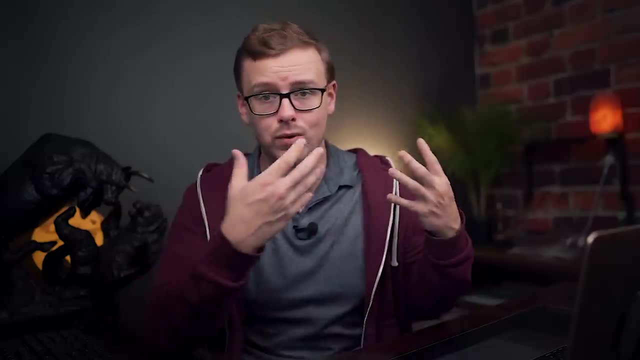 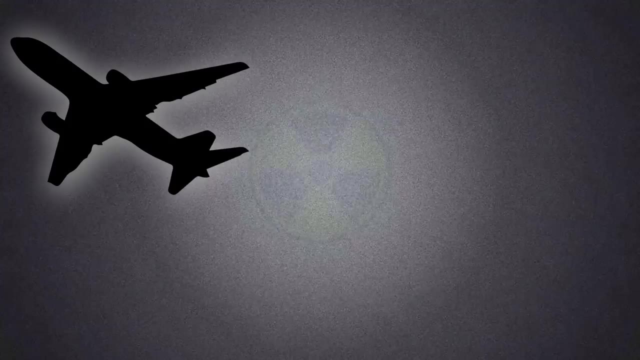 energy. other governments like this type of energy and they'll, you know, make regulations against this, But I personally think that nuclear energy is the future. I think a hundred years from now, uh, airplanes, cars, et cetera are all going to be running on the energy industry. 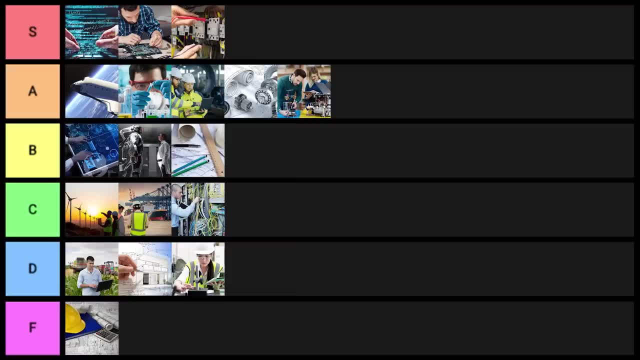 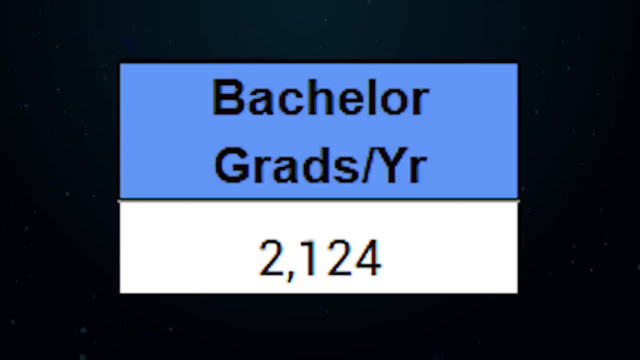 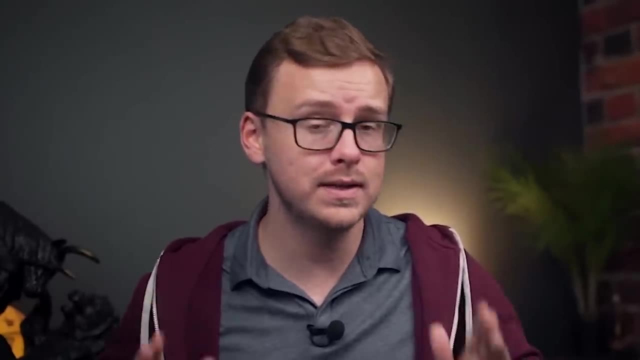 That's just my opinion, though, So for that reason, this one is going to go into C tier. Next one on the list is going to be petroleum engineering, with about 2000 graduates per year. Now, this is actually the highest paying degree period, Not just on this list, It's the highest. paying degree period. Yeah Wow, Early career pay. You start off $94,000 a year. Mid career pay is 176,000.. Absolutely So this is going to go into C tier. Next one on the list is going to be: 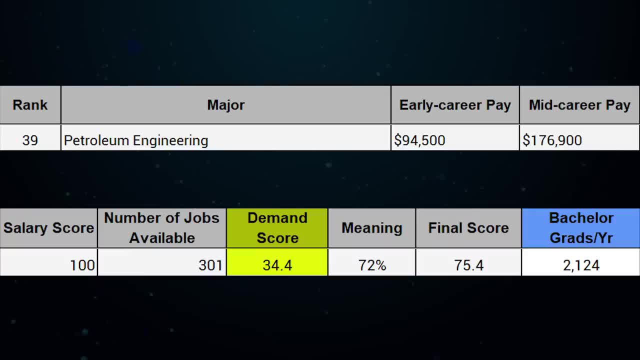 the highest paying degree period, Not just on this list, It's the highest paying degree period. It's the highest paying degree period, So this is going to be the highest paying degree period. However, the demand score is relatively low. It's only about 34. couple that with it not being a very